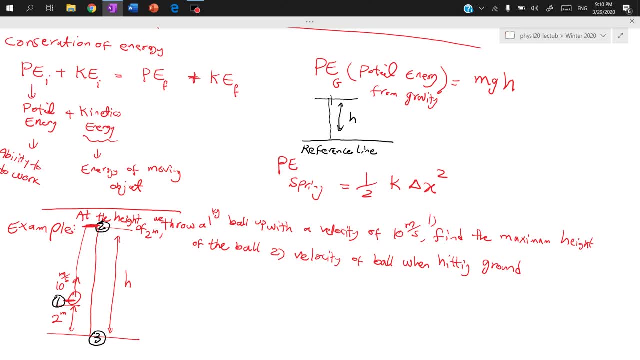 energy and then, or potential energy, initial plus kinetic energy. initial is equal to potential energy, final plus kinetic energy. final, as you can see the equation here. now, what is kinetic energy? that's what we talked before. kinetic energy is energy from motion, energy of moving objects, and potential energy is: 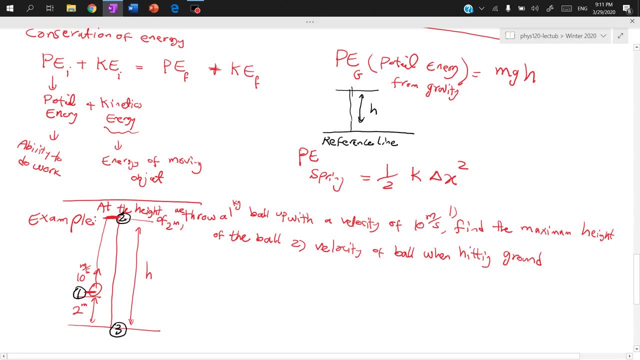 the ability to do work. so ability to do work. why? what do we mean by that ability to do work? not every time we can do work, so the ability to do work. for instance, if you have a ball which is 10 meter above the ground, that actually has the ability to do work. 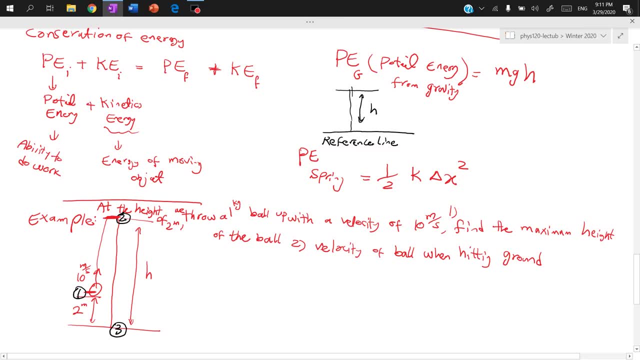 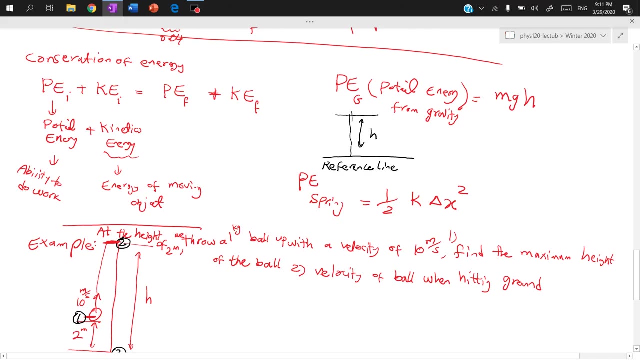 now potential energy. in physics we looking to two types of potential energy. one would be from gravity and the other one is from spring. so in order to calculate potential energy from gravity, we we need to have a reference line. in this case i put the ref. usually we put the reference line. 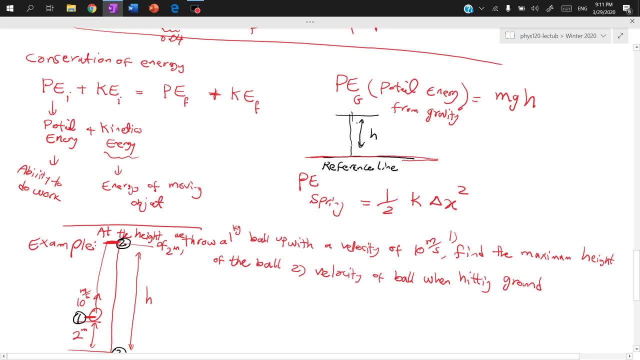 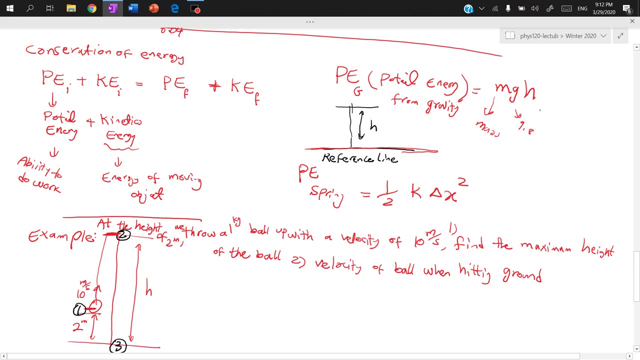 on the floor, on the ground, and then we look at the height that we have from the ground. so potential energy from gravity is mgh, where m is the mass, g is 9.8 and then h is the height above reference line. potential energy from spring is equal to half of k delta x to the power of. 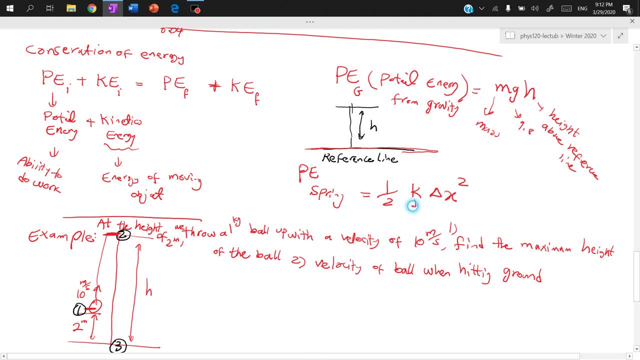 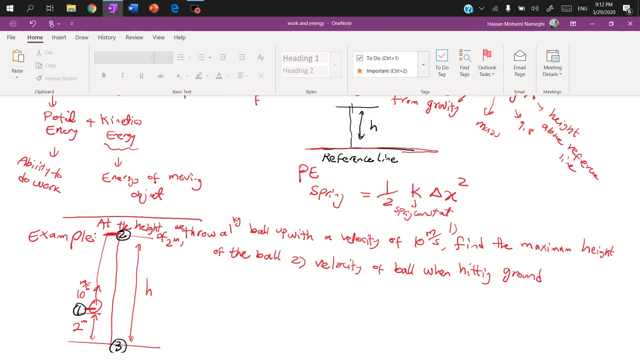 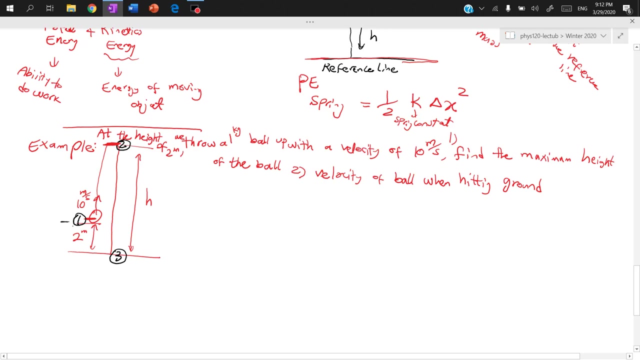 2. we already talked about that. k was spring constant. delta x is actually a stretch or compression on the spring. let's do a couple of examples. so in the first example i want to solve a ball. that ball actually through at point 1. we throw the ball up with 10 meter per second. the question asked was: find the maximum height where. the ball will go into. we know that as you go up, the velocity will reduce at the maximum height, where the velocity will be 0 for a second, the ball will start to go at a maximum crescent and only to that part of time we would actually reduce 1 meter per second. if that is, the maximum gonna be like 02 meter per second and we will now overcome this problem. so in summary, so when we come back to simple knowledge, i'm going to you repeat the following, one step by step: that jose did the, that first- выпela in a b. 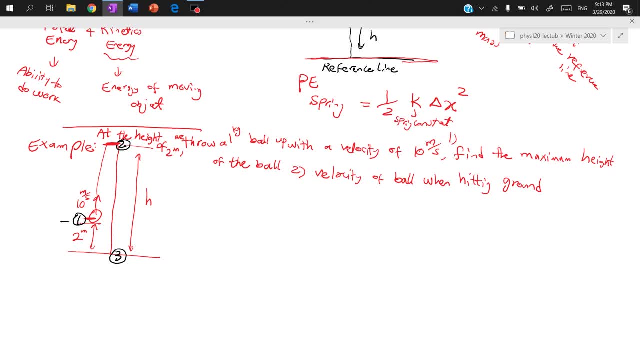 we know that as you go up, the velocity will reduce the maximum height. where the velocity would be 0 for a second, the ball will have zero velocity. then it go back. it will come back. the question: ask us to first to calculate the maximum height in which the ball can travel and then the second part of the problem ask us. 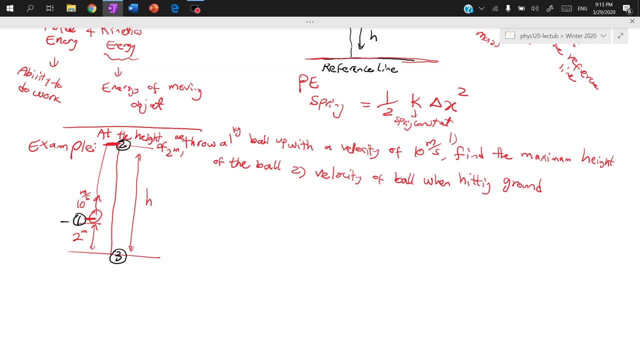 velocity of ball when it hitting the ground. so in this, to solve this problem, we need to have a reference line. so i'm going to first i'm going to solve part one. so for part one i have two points. i have point one and i have point two, so i can say potential energy one plus kinetic energy one. 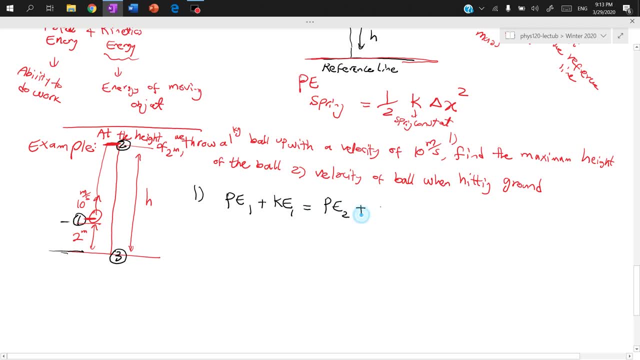 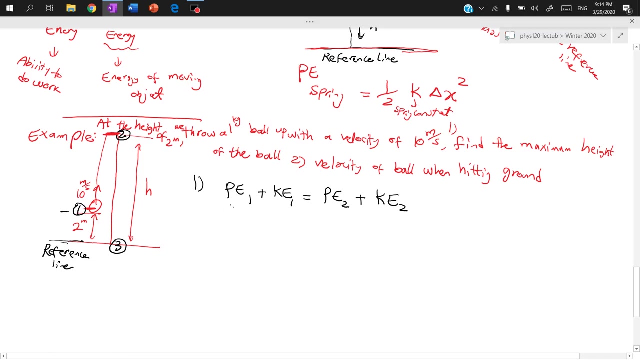 is equal to potential energy two plus kinetic energy two. now potential energy one. we need to have a reference line in this problem. i'm going to assume reference line as the, as the ground now the height above the ground is equal to. the height above the ground is two meter. so for p e one would be equal to m, g, h one. 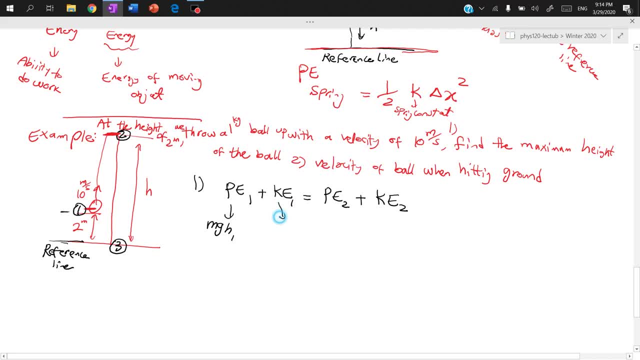 kinetic energy. one is half of m, v, one to the power of two, now h. one is two meter, g is 9.81. sorry, this course, we just use 9.8. so fs, e to infinity. and then the mass of the object is 1 kilogram. 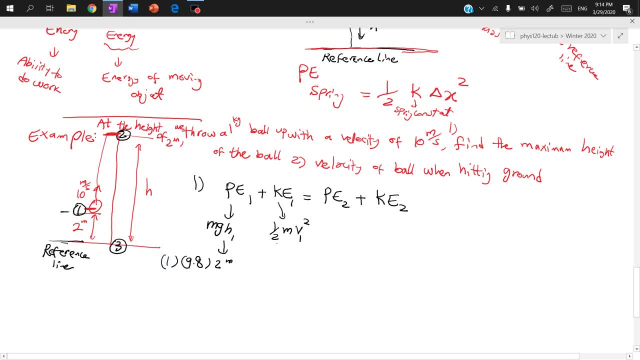 there you go. so this is potential energy for the first one, kinetic energy in the first situation. so we have plus half of one, and then v in the first position is actually 10 meter per second. so we are done with the first part of it. the second part, p e, 2. 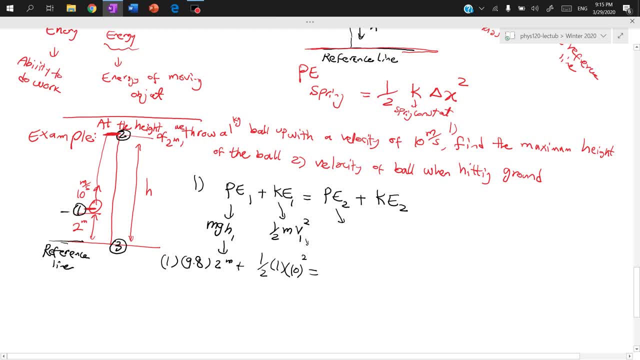 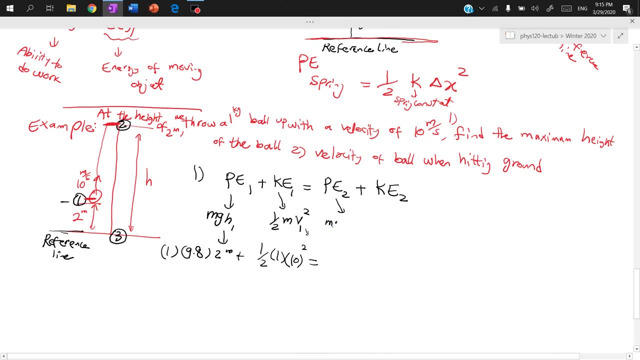 potential energy in position two. that's what we want to find. and then the third part is over here. what we want to find. we want to find how high this object will go into. so i'm going to call that m, g, h, that actually, that height is h. you can actually call it h2, but i just simply call 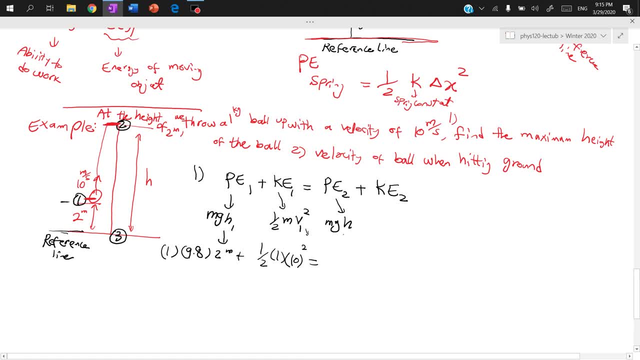 it h, because that's going to be easier. so then if you continue this, you're going to have 1, 0 square time plus k, e, plus t e i times 9.81 times 9.81 times h, plus ke2. so potential energy in. 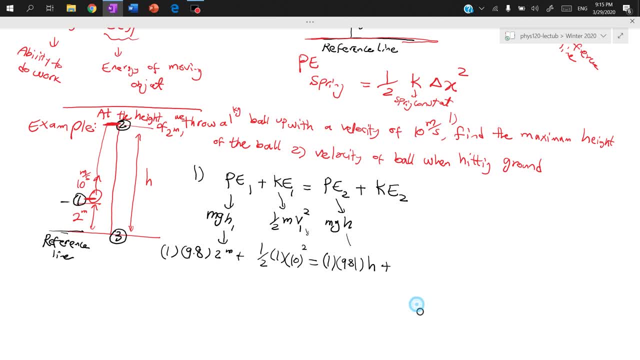 position two, sorry, kinetic energy in position two. position two is where the ball stops. so there the ball is stopped. if you say, half of the velocity will be zero. when the velocity is zero the kinetic energy is zero. so in this equation i want to solve for h, to find the value for h. 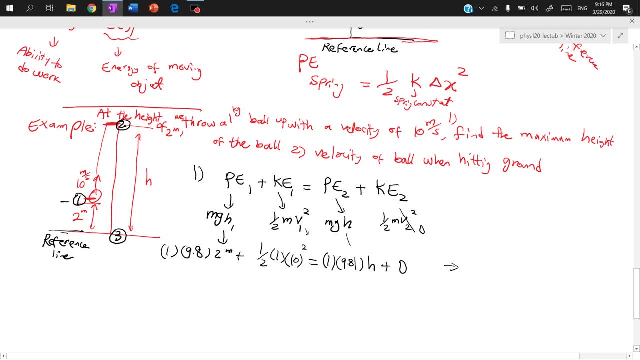 for h. you can. you can simplify this problem. if i simplify it, in one side i have 2 times 9.81 and then in the other side i have plus this. so this is actually is going to be 50. now i can bring that one to this side or to do to finalize the calculation there are. 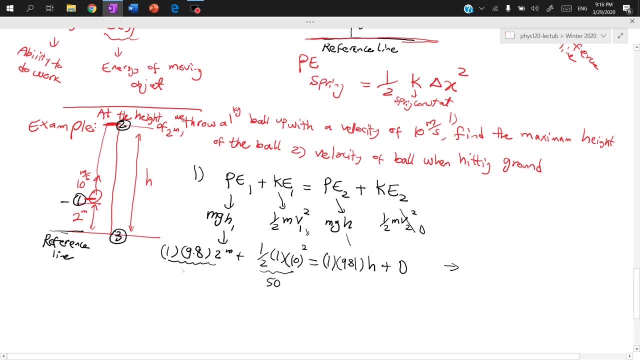 different ways to do that. if you simplify, here you're going to get 19.6 h down, here we're going to get 9.8 h. then i can solve for it. so i can say 9.8 h is equal to. now we have 50 and we have 19.6, so this will be 69. 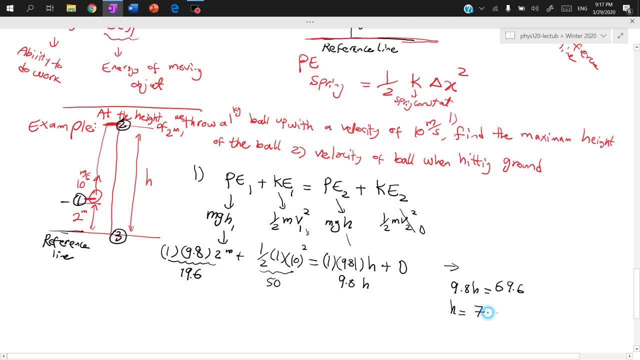 6, then if you solve for h, h will be equal to 7.1. if you divide both sides with 9.8- i'm sure you know how to do that- then you can find the value for for h. so you divide both sides by: 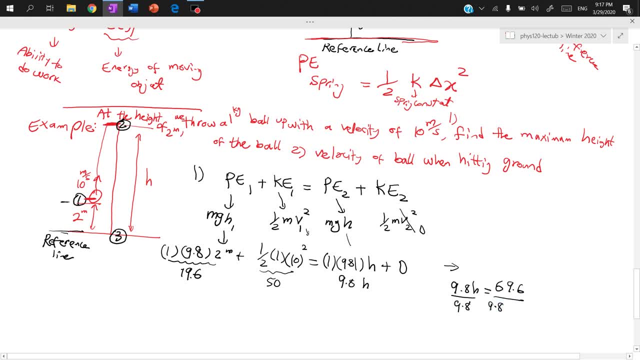 9.8, 9.8 and the value that you're going to get- you're going to get h- is equal to 7 point 1 meter. so the maximum height that this guy will go up will be 7.1 meter, part two. so 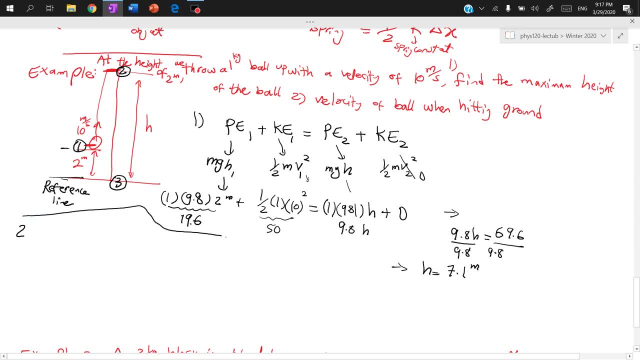 this is part one. part two: i'm going to draw a line to separate them. part two: the question asks me velocity of ball when hitting the ground. so when hitting the ground all the way, here you are at the reference line. your height will be zero. so let me just to set up the equation again: pe2 plus. 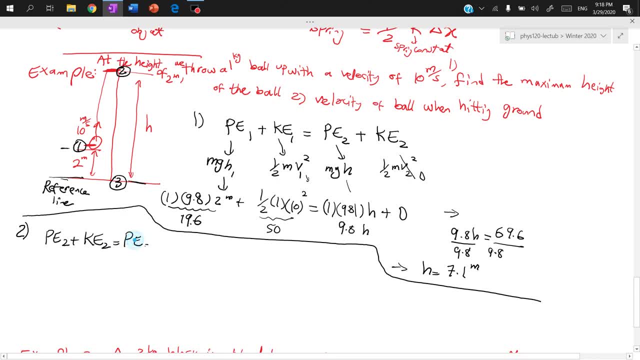 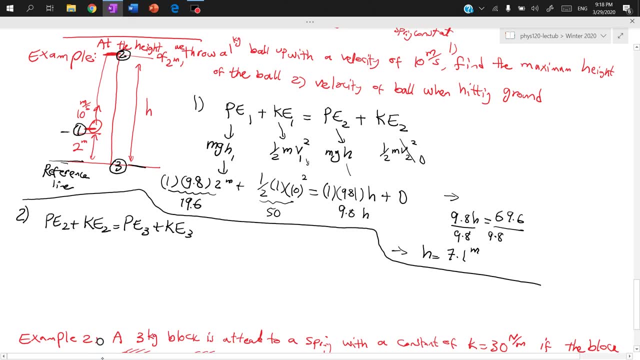 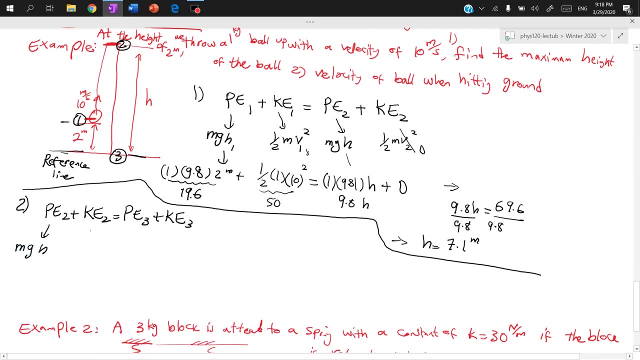 ke2 is equal to pe3 plus ke3, now pe2. at the position two we already calculate pu2, which was mgh. ke2 was zero. in position two, we have no kinetic energy, which was because the velocity was zero. in position three, potential energy is zero because when we say mgh, the value 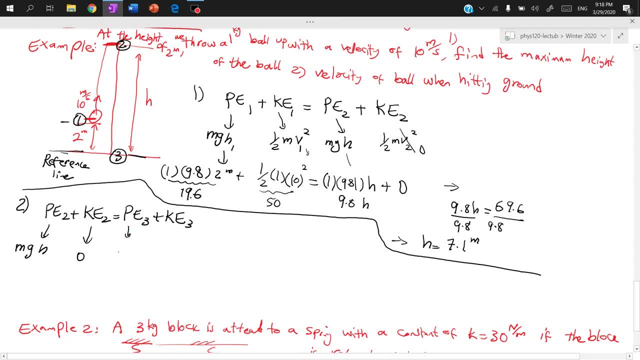 for h is zero, so this is actually mgh3, or h3 is zero, and then k3 is going to be plus half of mv3 to the power of two. so let's, let's do this. the calculation: the m is one kilogram, g is 9.8, h is 7.1. we got it from last time. 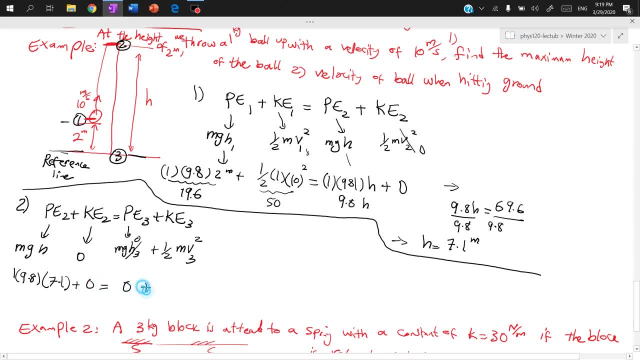 plus zero is equal to zero plus half of one times v3 to the power of two. then if i simplify this, i'm going to get v3 to the power of two is equal to two into. i'm just multiplied two side by two, two times 9.81, 9.8 times 7.1. 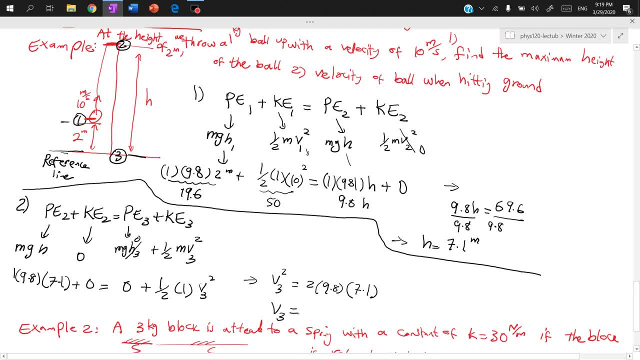 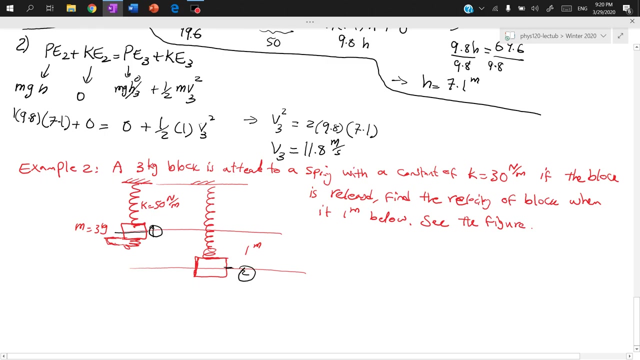 then if you simplify this you're going to get. v3 is equal to 11.8 meter per second. that's it. so we solved the first problem. second problem is a problem which is need a little bit more thinking. in this problem we have a block which is attached to a spring. spring is initially on on a stretch and then there's one. 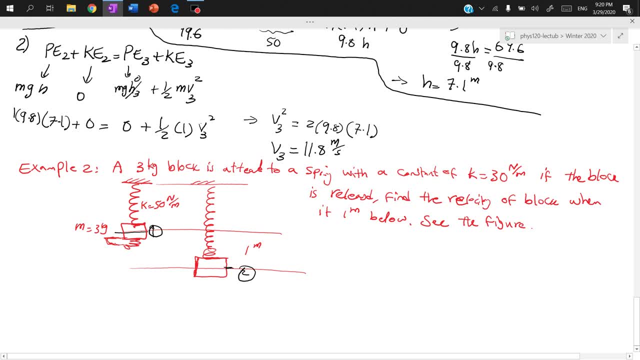 person is holding the spring, then we release our hand when we release overhand. the question asked us: when this spring is one meter below, calculate the velocity of just to the moment below therica to the position of the spring. desperate b means we needed to keep one meter below in the spring. 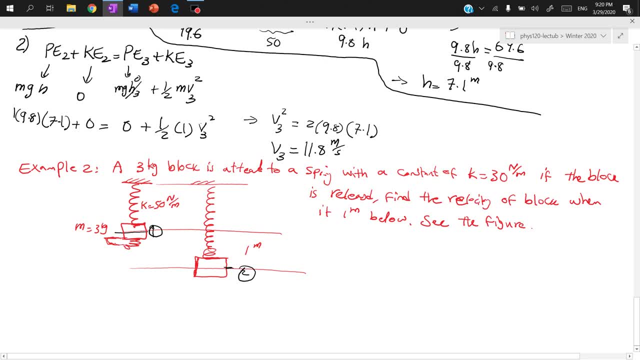 velocity of the block. so, in this case, position one and position two in position one. again, this is the vertical. they are in a vertical setting. in a vertical setting, we're going to have potential energy from gravity and then potential energy from the spring, so we have both potential energy. 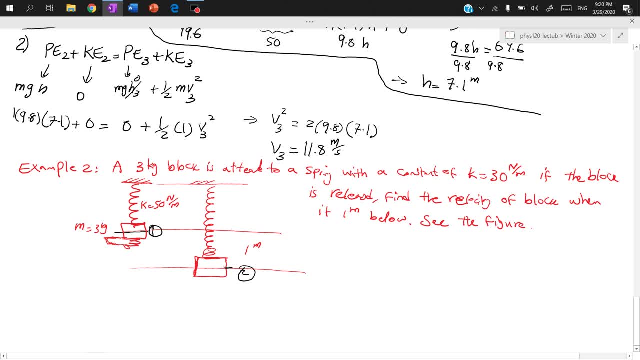 we need to find what is going on in position one, what types of potential energy we have in position two, what types of potential energy we have in position one, because we don't have any stretch from the spring, so we can say pe1 is equal to pe from g plus pe from. 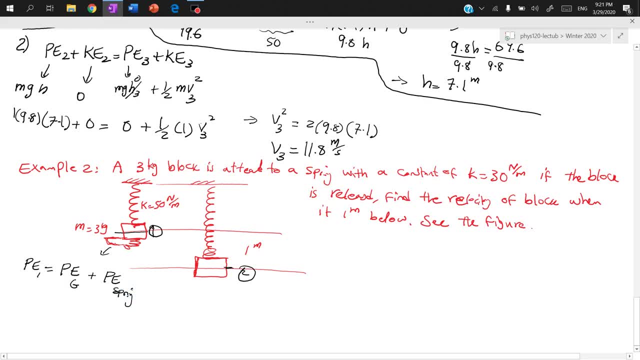 spring. so peg is actually is mgh. i'm going to assume the reference line down here: m is three kilogram, g is nine point eight and h. the value for h is simply one from a spring. so we already know the equation for a spring was half of k, delta x to the power of two. in the first position, spring doesn't have any. 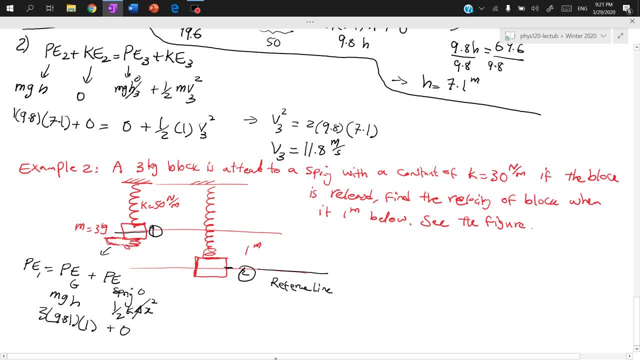 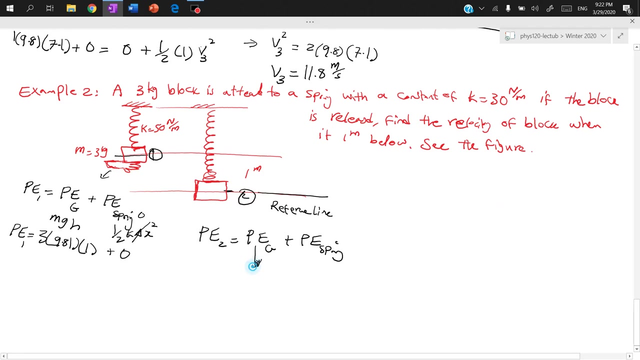 stretch. so this is actually zero. so it'll be zero. so this is how much pe1 is going to be. and in the position two, pe2 is equal to peg plus p from the spring. now, in position two, the height is zero. so therefore you can say: 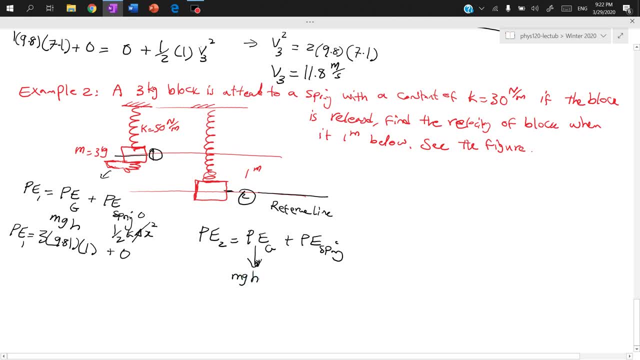 mgh, which h is zero. there is no height about the reference line, which is just the ground pe from the spring. so spring is actually already a stretch for the value of half of k. delta x to the power of two which we have. pe2 is equal to. that's what. that was: zero plus half of. 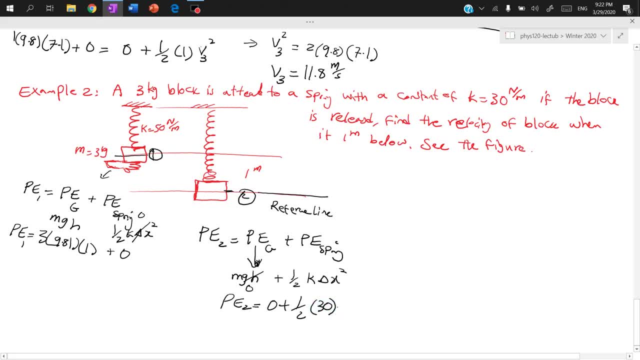 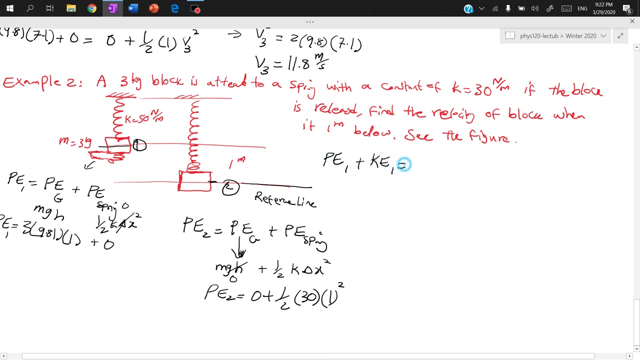 the value for k, which is 30, delta x is one meter. you can see that it's been stretched for one meter to the power of two. now, in the beginning, because we say we release it in position one, your kinetic energy is zero. so let me just to list the rest of them. we know that pe1 plus ke1 is equal to pe2 plus. 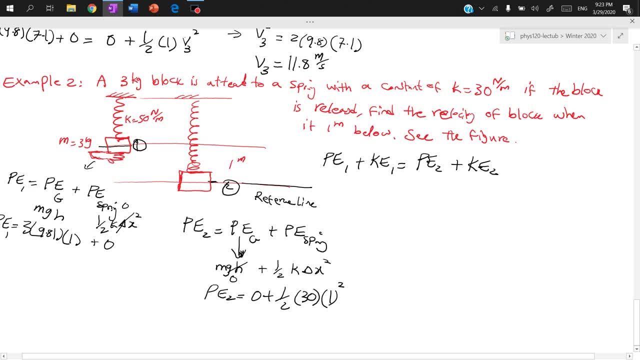 kinetic energy plus potential energy stay constant. the sum of it so potential energy plus kinetic energy is equal to potential energy plus kinetic energy. so potential energy in position one. we already know that that's actually three times nine, point eight to times one, which i don't consider the one. kinetic energy in position one. 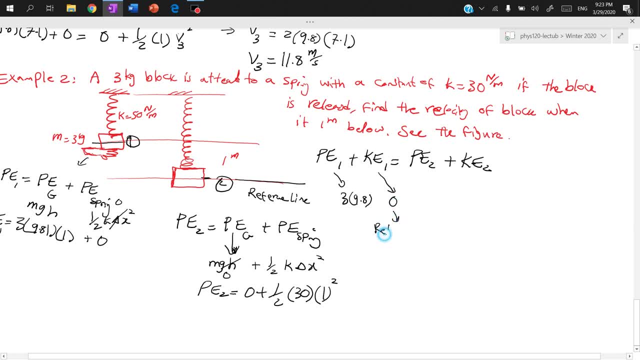 will be simply zero because we release it. when you release it, velocity is zero and kinetic energy will be zero. potential in the position two is going to be half of 30.. again, one to the power of two will be one kinetic energy in the position two, which is half of. 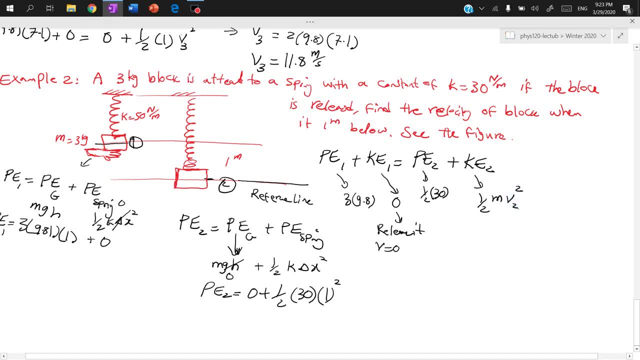 mv to the power of v2 to the power of two, so now m is three and then we can calculate it. so this will be this plus this is equal to this. so i have- i'm going to simplify this equation- i have 3.3 times. 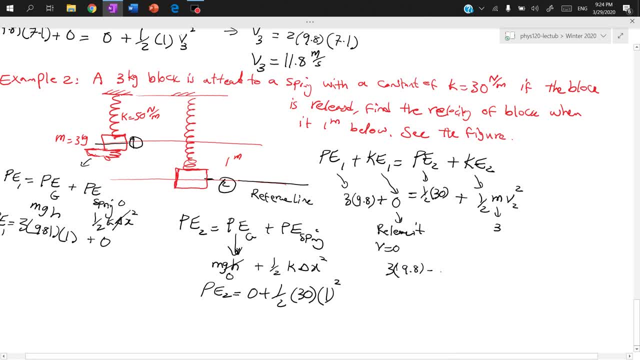 9.8 minus half of 30, which is 15.. i will just simply put here: half of 30 is equal to half of 3 kilogram into v2, to the power of 2.. now you simplify this side. when you simplify this side. 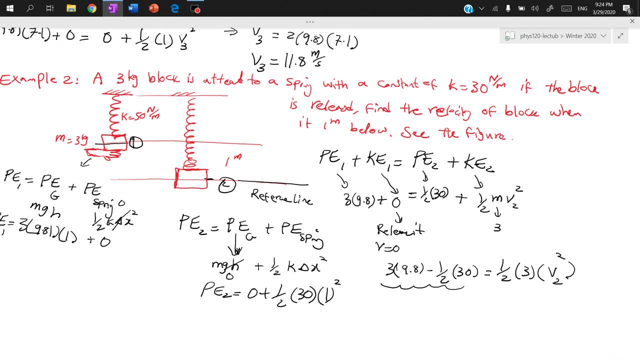 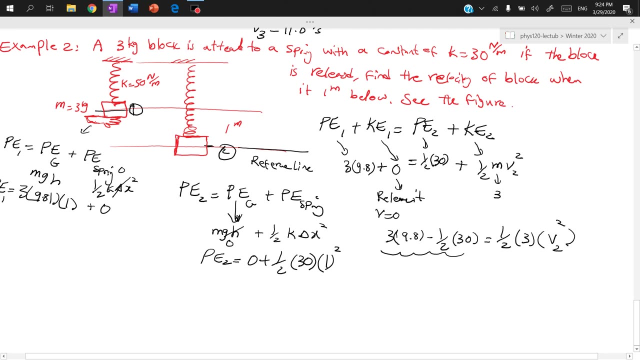 you're going to get 14, point 14.48, 14.86. then you can simplify the other side too, which we have like 3 over 2, which would be 1.5. then you can solve for the value for v2 and then that value for. 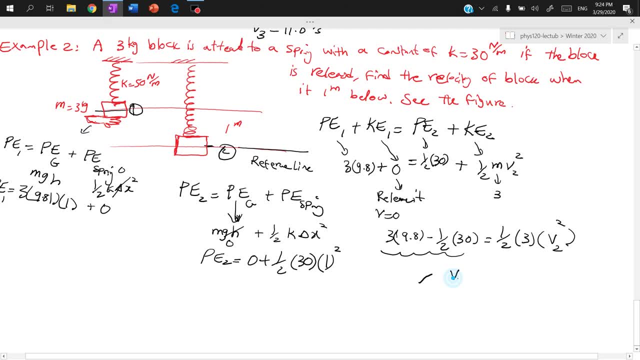 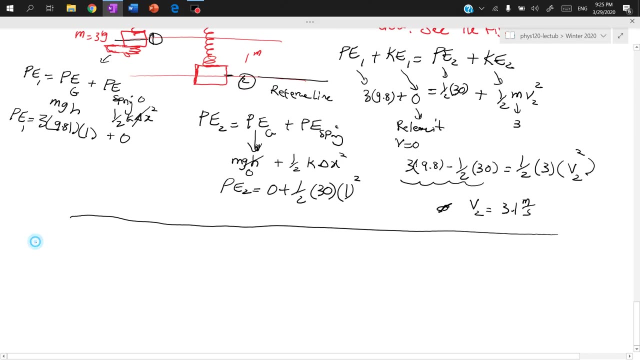 v2. i got it here as the value for v2. i got that 3.1 meter per second. now the very much to the end of this lecture. we talk about power. power meaning that work over time. so work overtime. what do we mean? work overtime if something done.